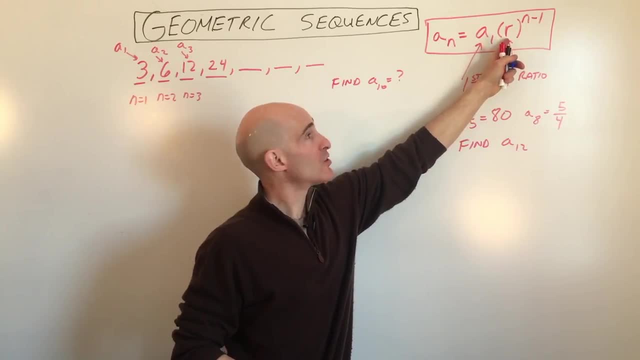 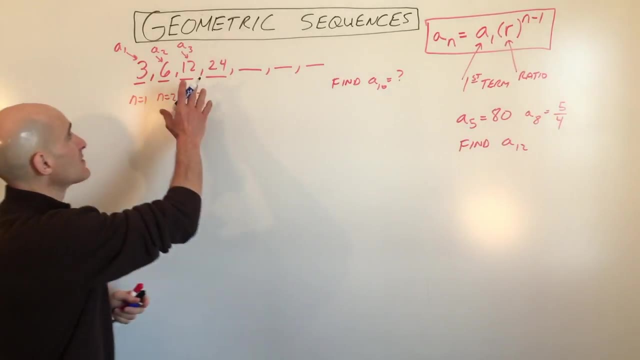 1 is the first term, r is the ratio. what you're multiplying by n is whatever term you want to find. So, if you want to find the tenth term, n equals 10 and so on. So, going back to this example, here we're starting at 3 and you can see, n equals 1 means this. 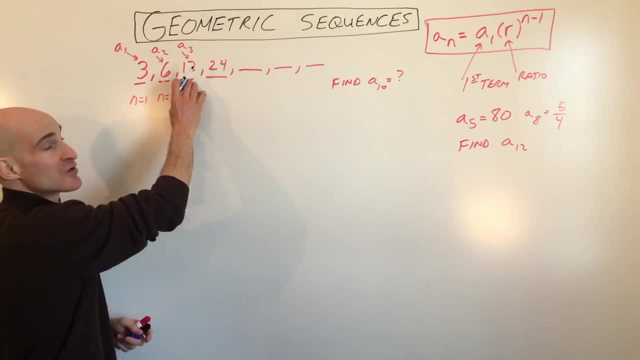 is our first term. n equals 2, that means it's the second term. n equals 3 is the third, and so on. But a sub 1 means that's the value of the first term. a sub 2, see this- is a. 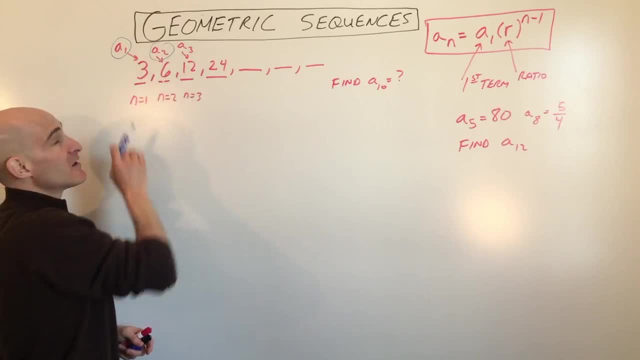 little subscript. it just tells you that that's the term. you're on the second term, the value of that term is 6, and so on. So if we wanted to find the, let's see 1,, 2,, 3,, 4,. fifth, 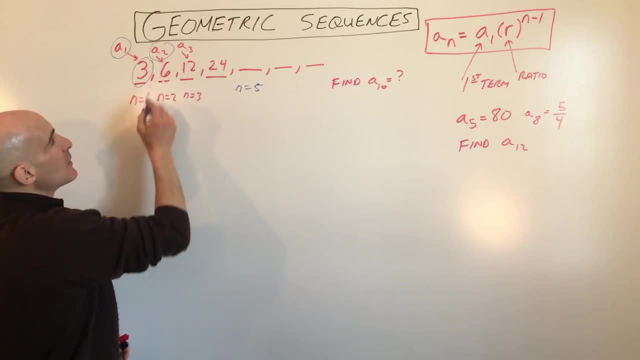 term okay n equals 5.. We would start at 3.. Okay, Okay, Okay, Okay, And we would multiply by 2, once, twice, 3 times, 4 times Okay, why not 5 times? Well? 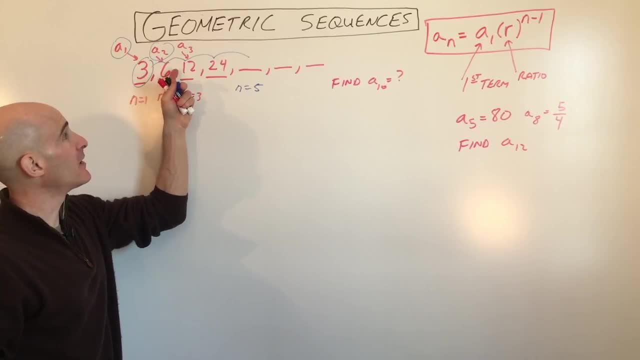 we already started at 3, the first term, so we only had to multiply by the common ratio to one less number of times. Okay, because we were already here, we just took 4 times. that's where the n minus 1 comes from. And now the ratio. why do they call it a ratio? 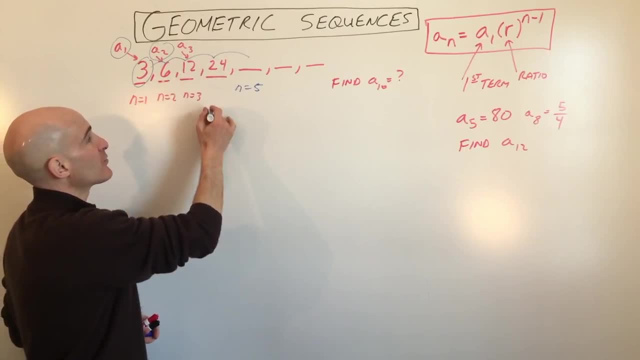 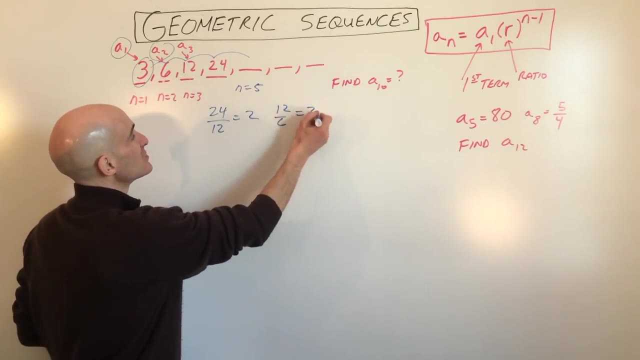 They call it a ratio, because if you take this number, this term, and you divide it by the first one, it will be 4, divided by 12 equals 2.. 12 divided by 6 equals 2.. And 6 divided by 3 equals 2.. So if you take the term divided, 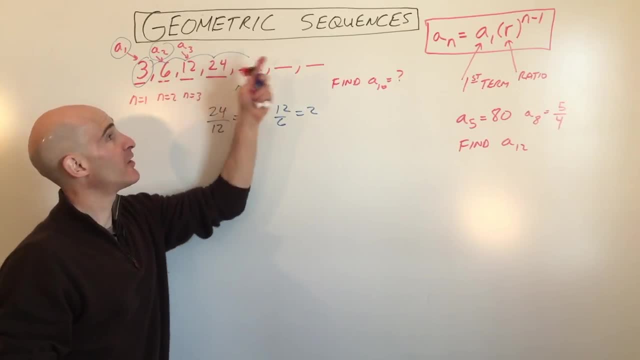 by the one before it. that gives you the ratio and that's what you're multiplying by to move forward to the next term, and so on. So say, we want to find the tenth term. well, we could keep multiplying by 2, okay, which? 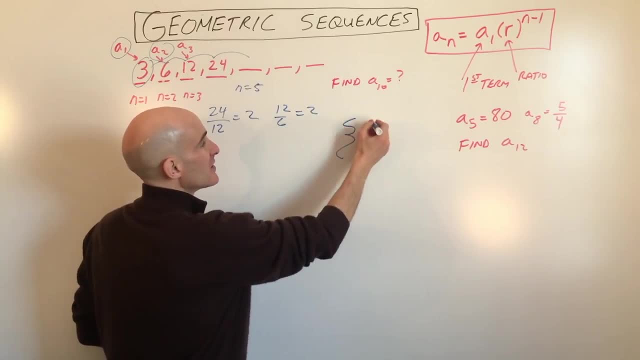 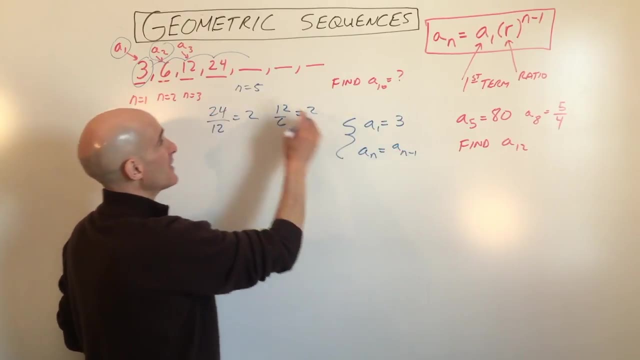 that's one way to do it. that's a recursive way. That would be like this: a sub 1 equals 3.. a sub n equals 2.. 1 equals 2.. a sub n minus 1. that just means you go back to the previous term and you add: 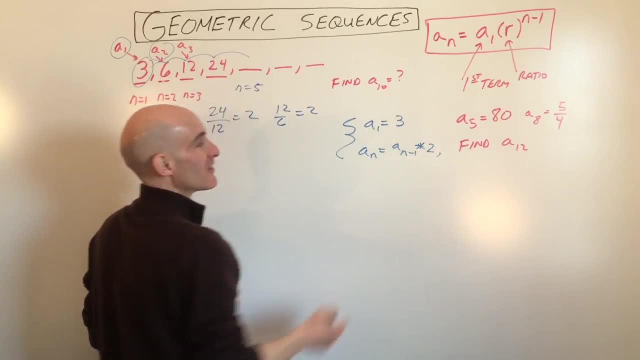 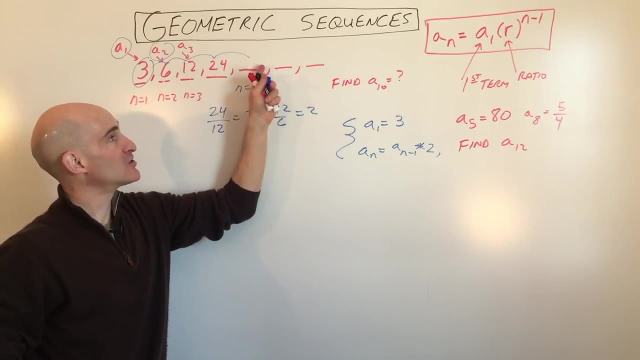 not add. in this case you're multiplying by 2, right? okay? so that's a recursive way to write the formula. you keep going back one term, see n minus 1, and then you multiply by 2. if you want the sixth term, you go back to the 6 minus 1. the fifth 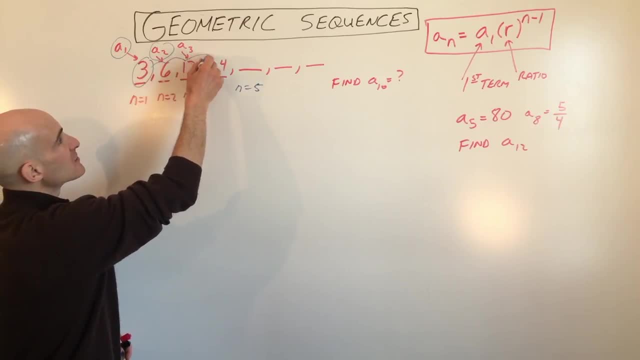 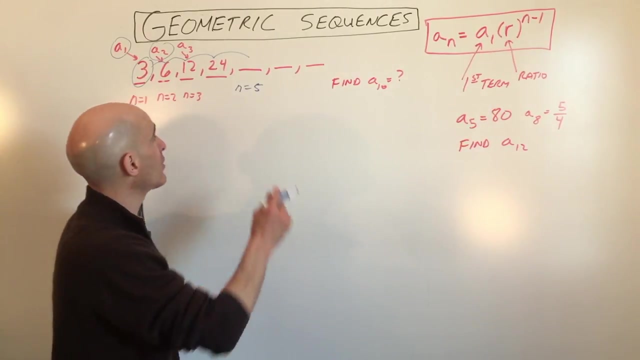 and we would multiply by 2 once twice, 3 times, 4 times. Okay, why not 5 times? Well, we already started at 3, the first term, so we only had to multiply by the common ratio to one less number of times. okay, because we were already here, we just took 4 times. that's where the n minus 1 comes from. And now the ratio. why do they call it a ratio? They call it a ratio because if you take this number this term and you divide it by the previous term, 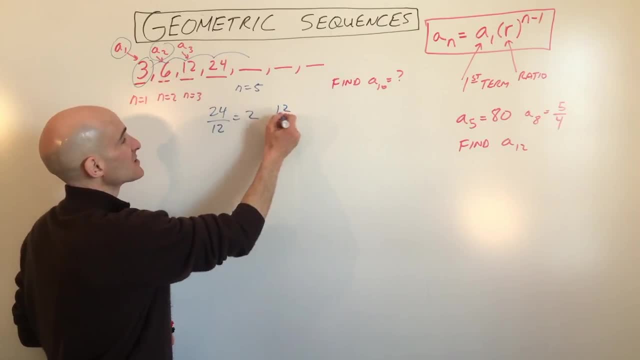 4 divided by 12 equals 2,, 12 divided by 6 equals 2, and 6 divided by 3 equals 2.. So if you take the term divided by the one before it, that gives you the ratio and that's what you're multiplying by to move forward to the next term, and so on. 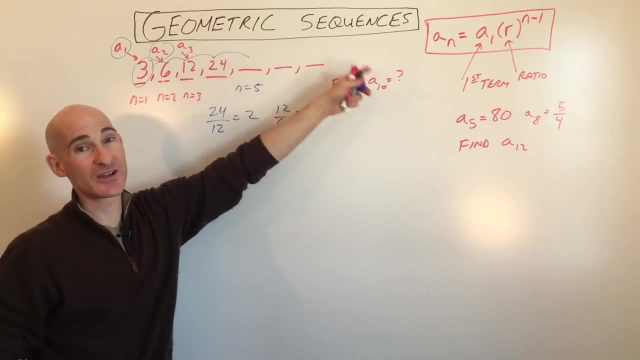 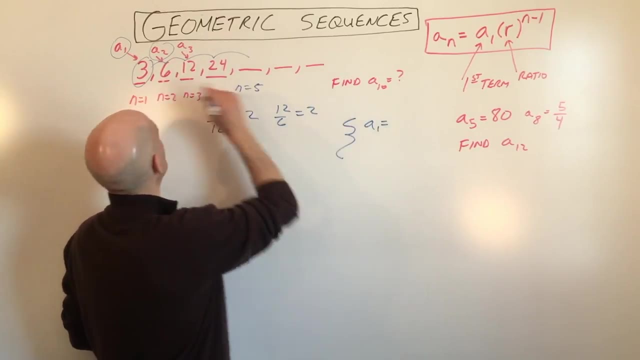 So say, we want to find the 10th term. well, we could keep multiplying by 2, okay, which? that's one way to do it. that's a recursive way. that would be like this: a sub 1 equals 3, a sub n equals a sub n minus 1, that just means you go back to the previous term and you add, not add. in this case, you're multiplying by 2, right. 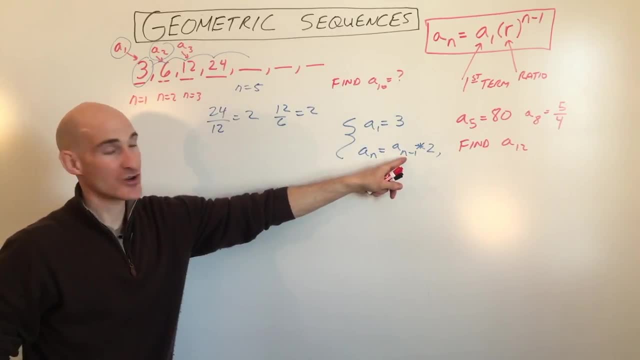 Okay, so that's a recursive way to write the formula. you keep going back one term- see n minus 1, and then you multiply by 2.. If you want the 6th term, you go back to the 6 minus 1,, the 5th term you multiply by 2.. 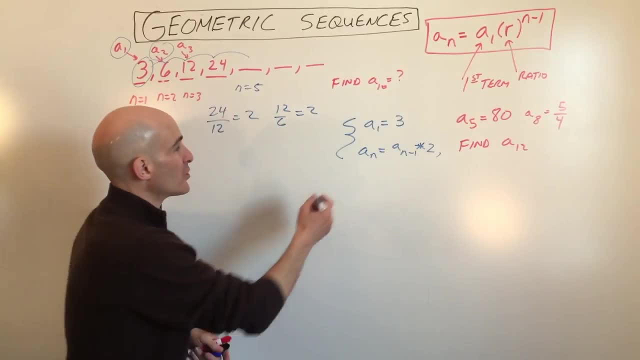 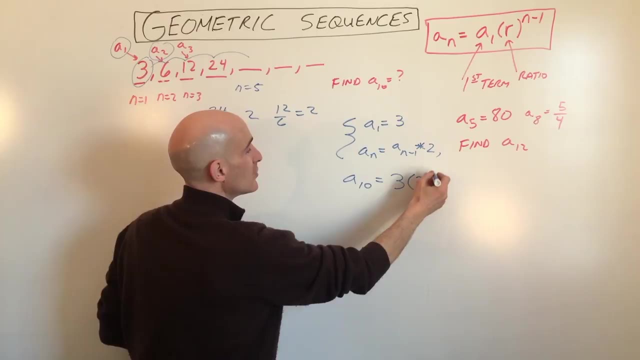 But this is an explicit formula that takes you right there, and so what you have is: you have the tenth term. So we start off with the first term, which is three. We're multiplying by two, nine times, because we're already at three. to get to the tenth term, We just have to multiply one. 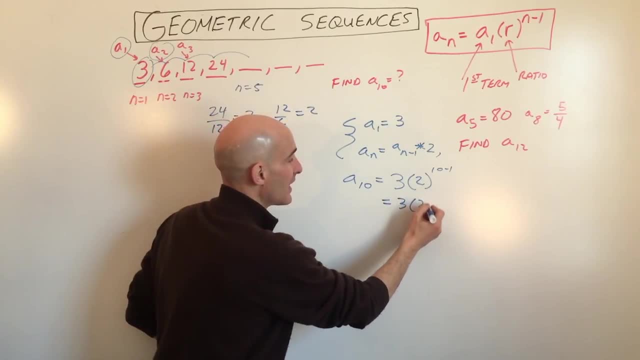 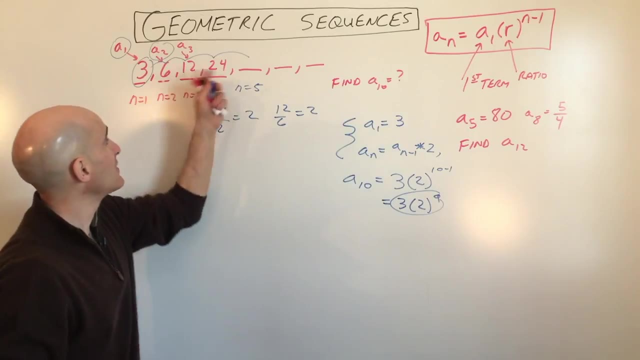 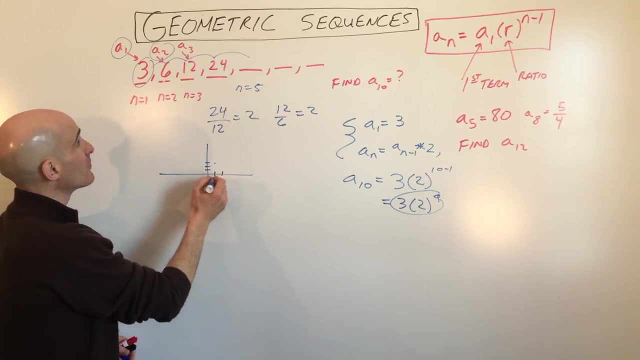 less time, And so this is just going to be three times two to the ninth. That's the value of the tenth term. Now, if you were to plot these points like if we were to draw this on a coordinate axis, So term number one is three, Term number two is six. Term number three is: 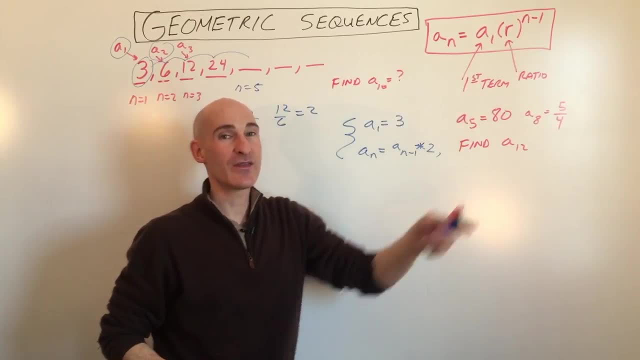 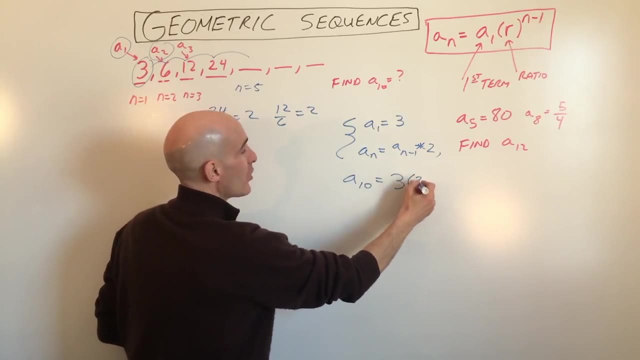 term, you multiply by 2, but this is an explicit formula that takes you right there, and so what you have is: you have. we want to find the tenth term, so we start off with the first term, which is three. we're multiplying by two nine times, because we're already at three. to get to the tenth term, we just have to. 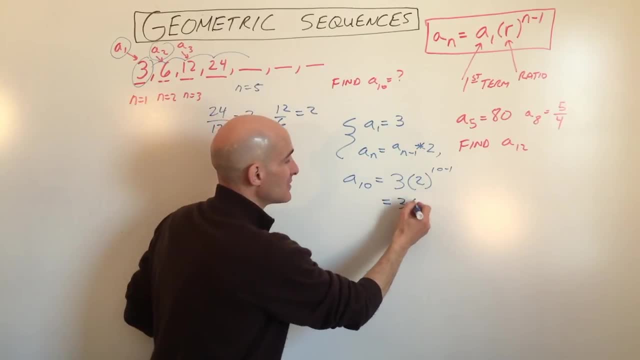 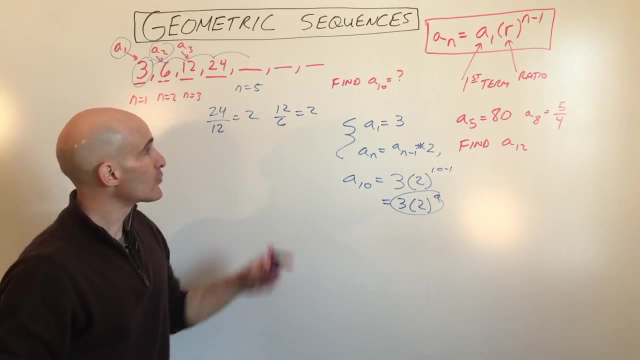 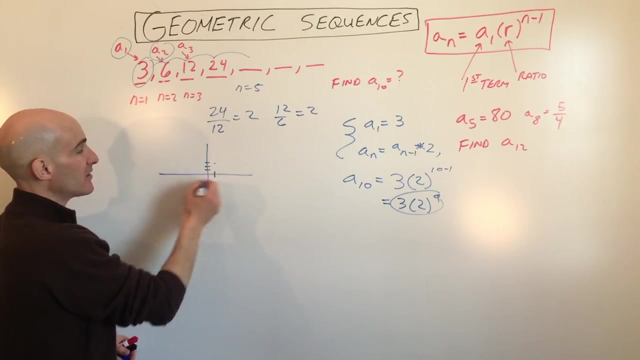 multiply one less time, and so this is just going to be three times two to the ninth. that's the value of the tenth term. now, if you were to plot these points like we were to draw this on a coordinate axis. so term number one is three term. 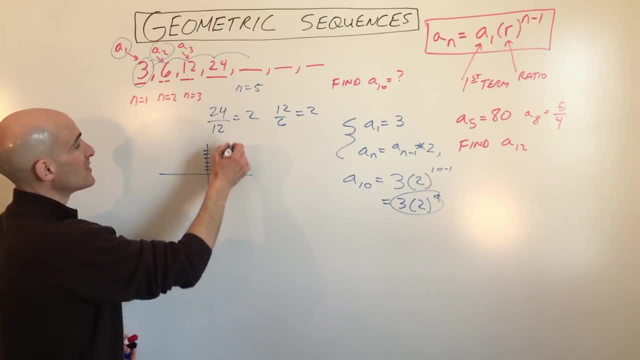 number two is six. term number three is seven, number three is 12. And if you can see this, it's going up at a faster and faster rate. This is actually an exponential curve, Whereas when we did the arithmetic ones it was linear, It was. 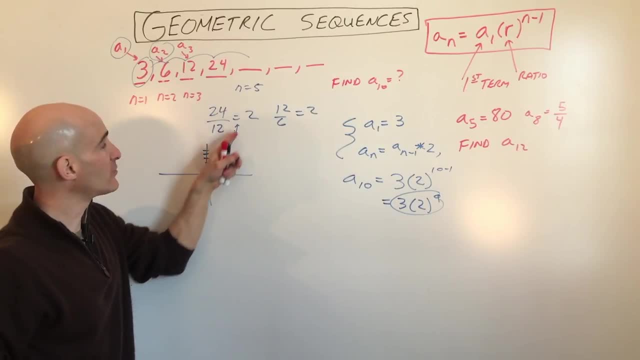 going up at a constant rate. You kept adding that common difference. Here we're multiplying by the ratio And you can see it looks like an exponential equation. The variable is in the exponent. Okay, so that's how you work with this. when they give you a list, Well, what happens if they just 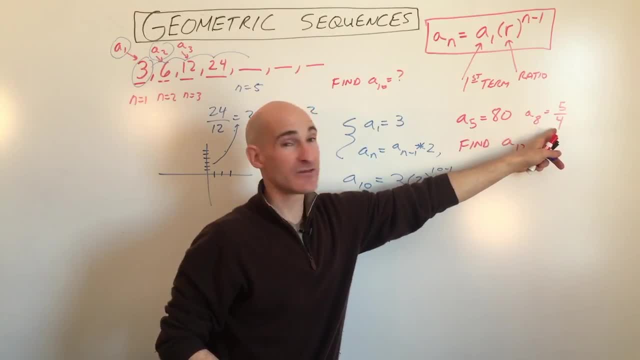 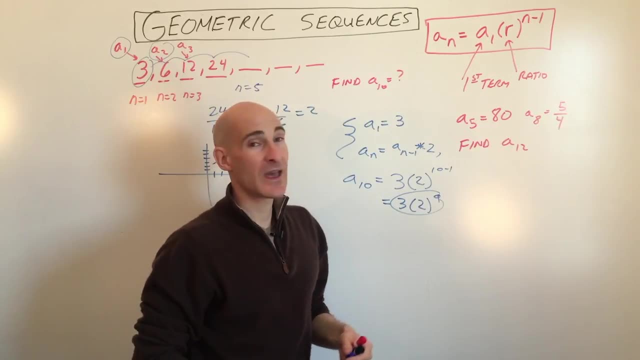 give you two terms, like the fifth term is 80 and the eighth term is five fourths. They tell us it's a geometric sequence, but find the 12th term. Hmm, how do we handle that? Well, what we're going to. 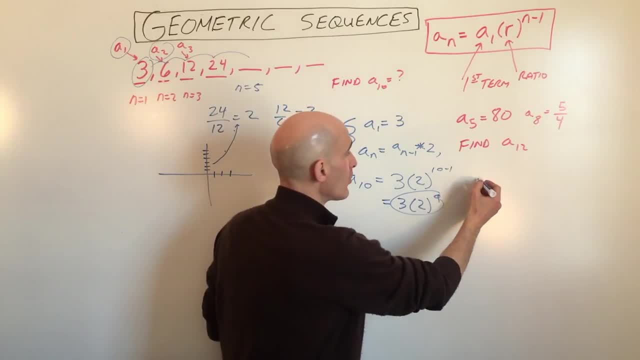 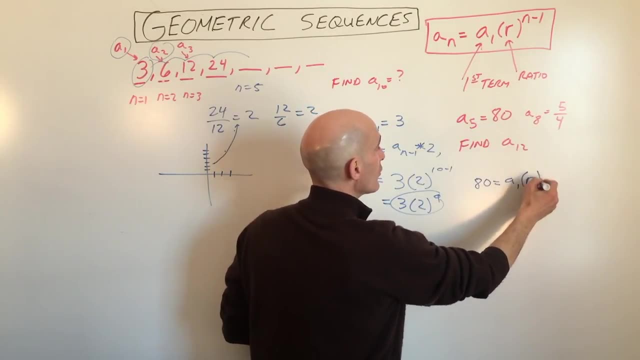 do is we're going to write a system of equations. So what we're going to do is we're going to say the fifth term is 80. The first term, we don't know The ratio, we also don't know But five minus. 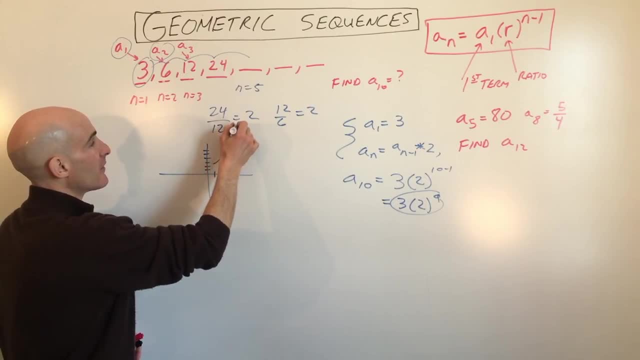 twelve And, if you can see this, it's going up at a faster and faster rate. This is actually an exponential curve, Whereas when we did the arithmetic ones it was linear. It was going up at a constant rate. You kept adding that common difference. Here we're multiplying by the ratio. 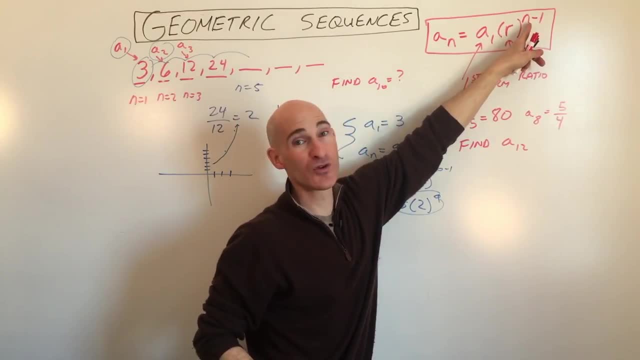 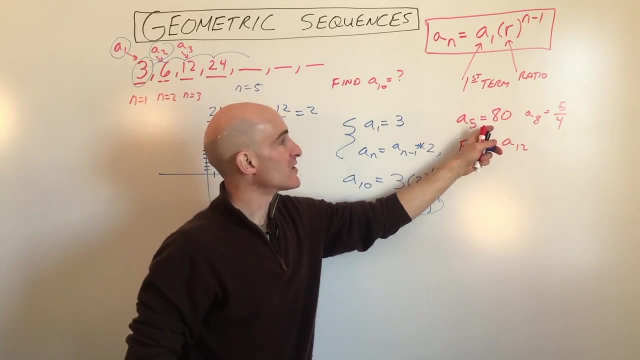 and you can see it looks like an exponential equation. The variable is in the exponent. Okay, so that's how you work with this. when they give you a list, Well, what happens if they just give you two terms, Like the fifth term? 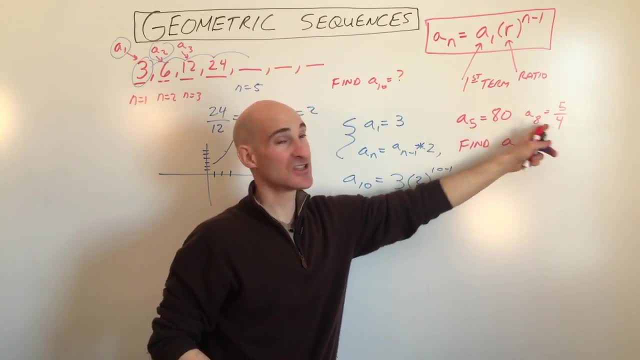 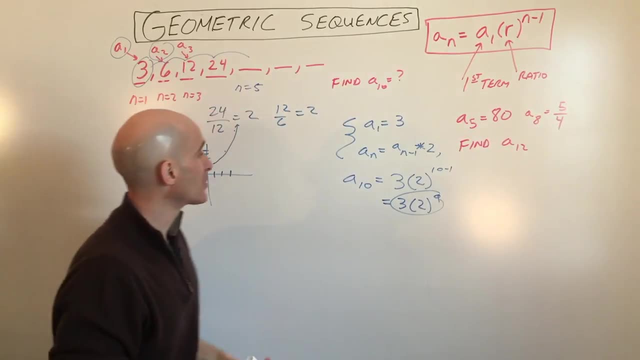 is 80 and the eighth term is five-fourths. They tell us it's a geometric sequence, but find the twelfth term. Hmm, how do we handle that? Well, what we're going to do is we're going to write a. 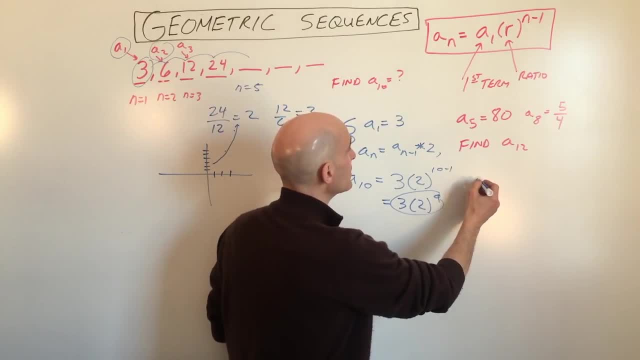 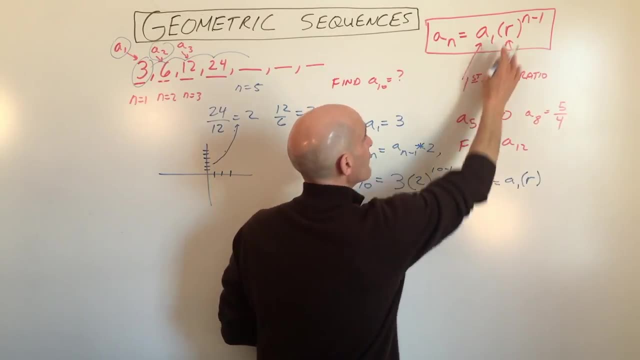 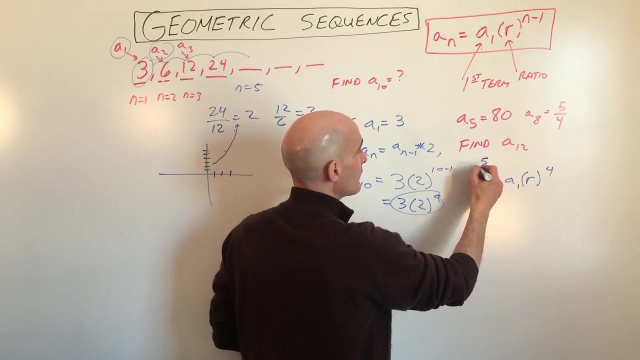 system of equations. So what we're going to do is we're going to say: the fifth term is 80.. The first term, we don't know The ratio, we also don't know. But five minus one is four. Okay, then we're going to say, all right, the eighth term. So the eighth term is five-fourths. 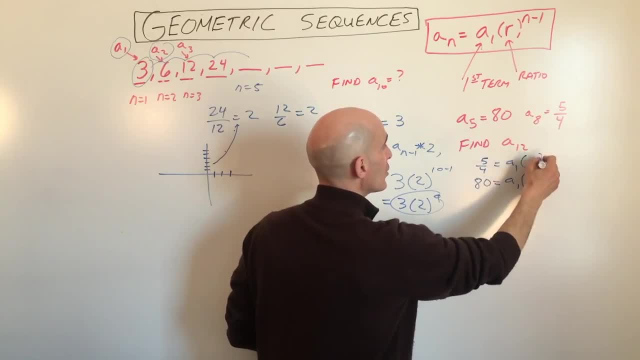 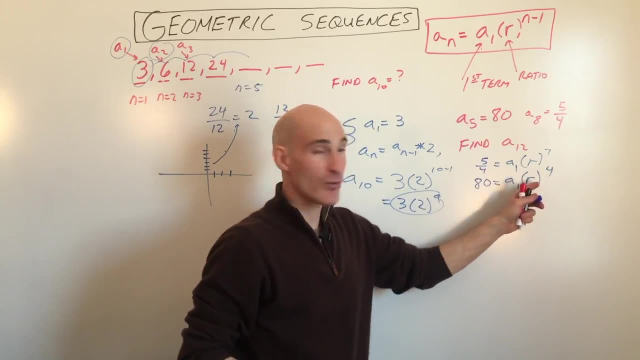 We don't know the first term, We don't know the ratio, but we know that eight minus one is seven. So now we have two equations, okay, two variables, and we can solve that system. So what we're going to do? 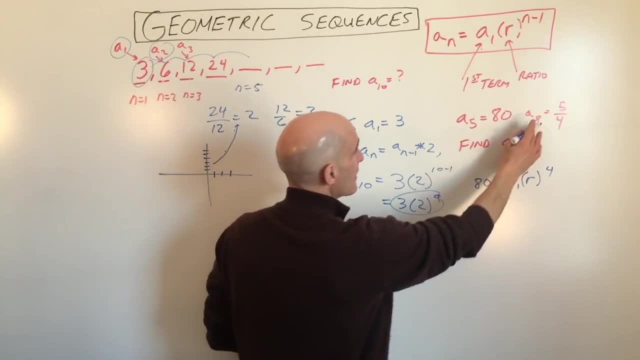 one is four. Okay, then we're going to say, all right, the eighth term, So the eighth term is five. And then we're going to say, all right, the eighth term is four. And then we're going to say: 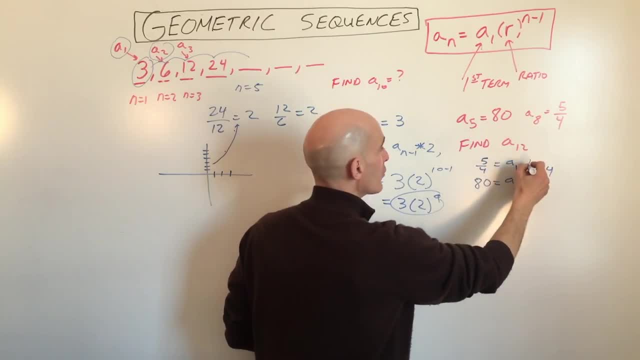 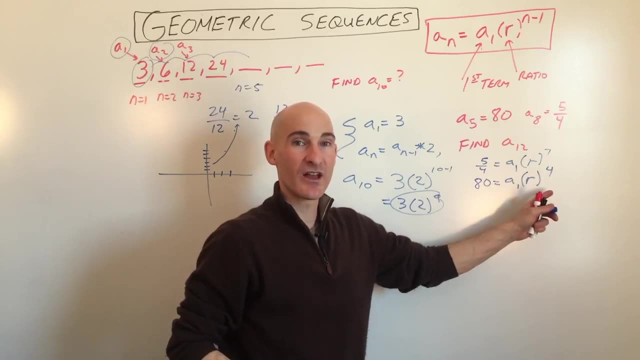 five, fourths. We don't know the first term, We don't know the ratio, But we know that eight minus one is seven. So now we have two equations, okay, two variables, and we can solve that system. So what, we're going to do something maybe a little bit different than you've seen before. 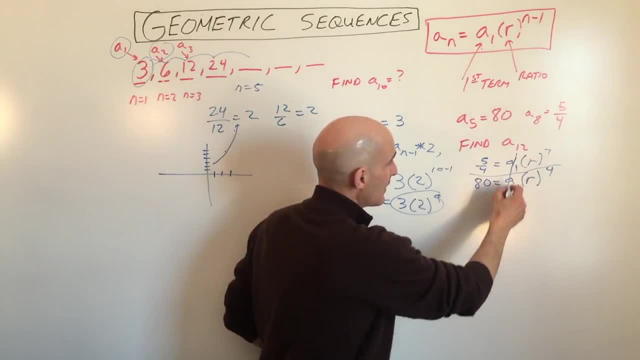 we're going to actually divide. So when we divide, see how the a ones cancel one another out. Seven minus four: when you divide and you have the same base, you subtract the exponents. Remember that. So it's r cubed equals. 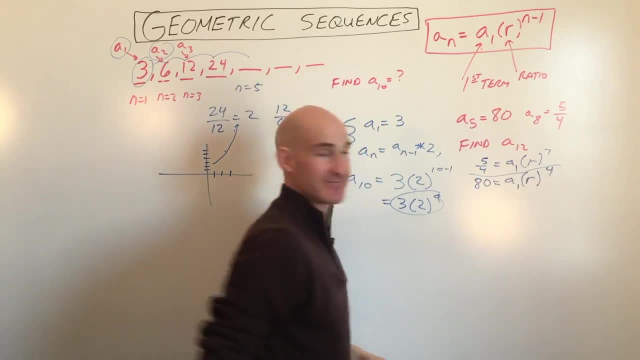 something maybe a little bit different than you've seen before. we're going to actually divide. So when we divide, see how the a1's cancel one another out. Seven minus four, when you divide and you have the same base, you subtract the exponents. Remember that. 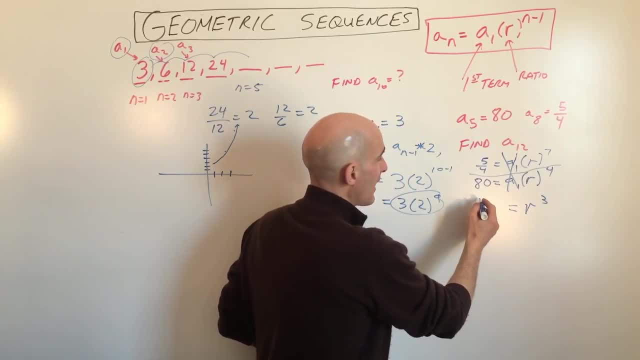 So that's r cubed equals five-fourths divided by 80. When you divide by a fraction, it's like multiplying by the reciprocal. So this is five-fourths times 180.. I'm going to reduce. Five goes in here once. Five goes in here 16 times. 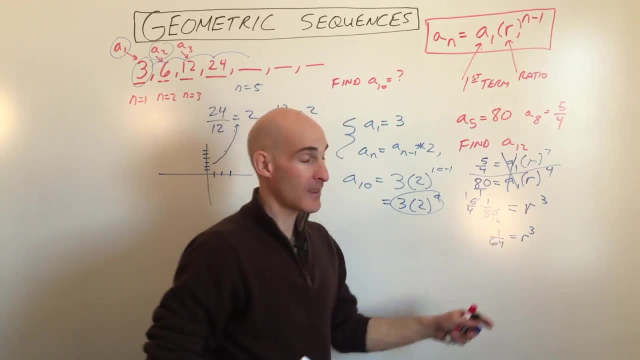 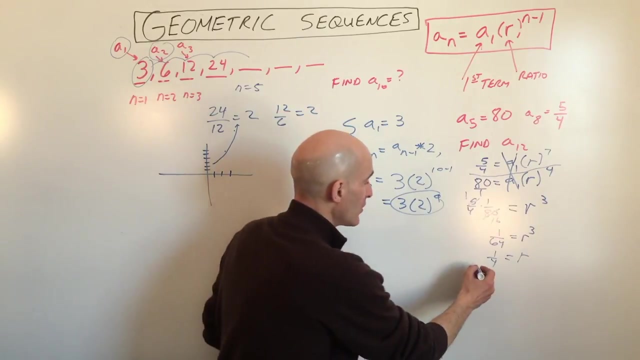 So this is one-sixty-fourth equals r cubed. If you take the cube root of both sides, you can see that r equals one-fourth. Okay, So now we know the ratio. If we put it back in to any one of these equations, maybe I'll just put it back into this one right here.